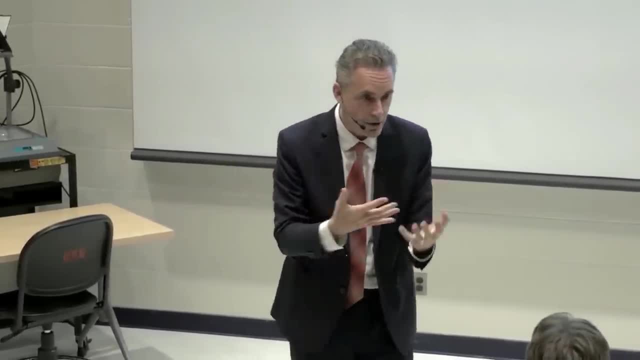 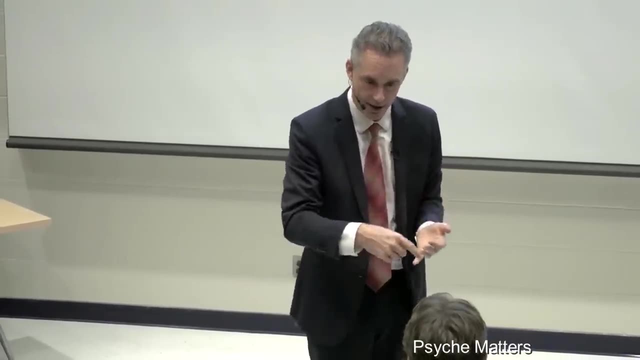 Well, let's talk about friendships for a minute. Here's how you know if someone's your friend A You can tell them bad news and they'll listen. They won't tell you why you know you're stupid and why that bad thing happened to you and how something worse happened to them once and you know. 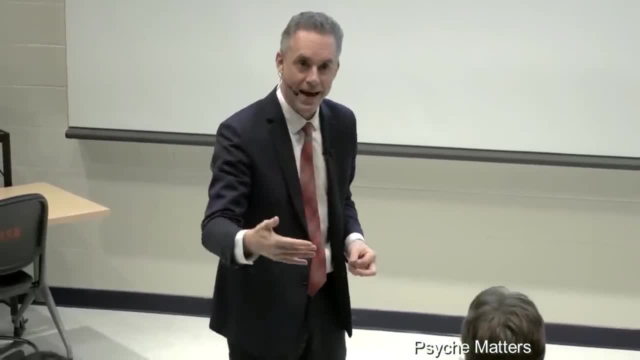 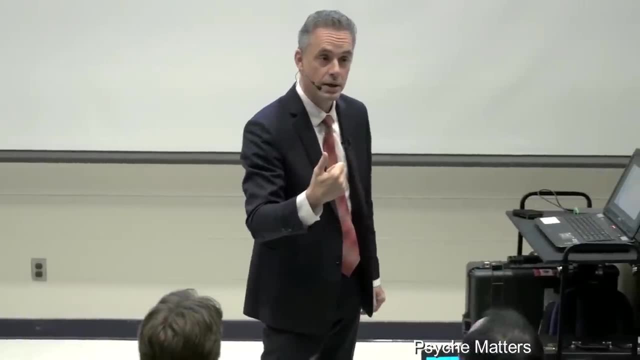 derailed the whole conversation. You can actually tell them bad news and they'll listen, So that's a good thing. And then- this is a weirder thing- You can tell them good news and they'll help you celebrate, And that's a really good way of deciding who you should have around you, Because 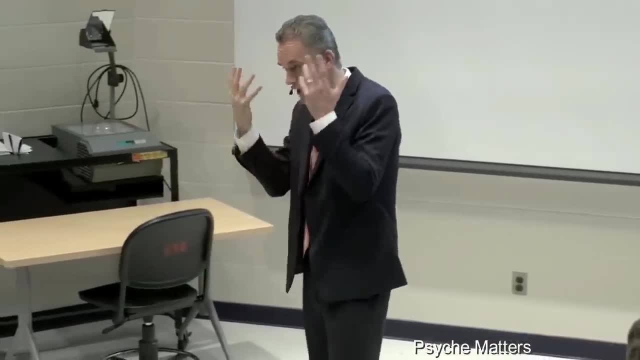 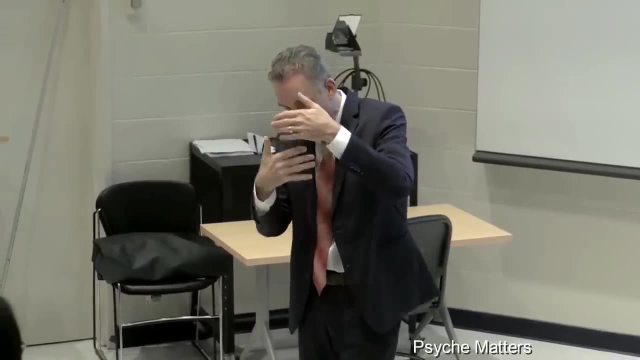 if you have someone around you, you know something good happens to you and you're kind of afraid to even admit it because you know God, something good happened to you. It's like you let that be known and it'll certainly be taken away. So you know, you come out and you sort of tell someone. 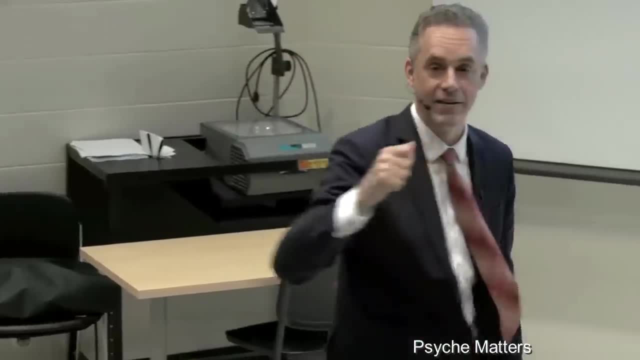 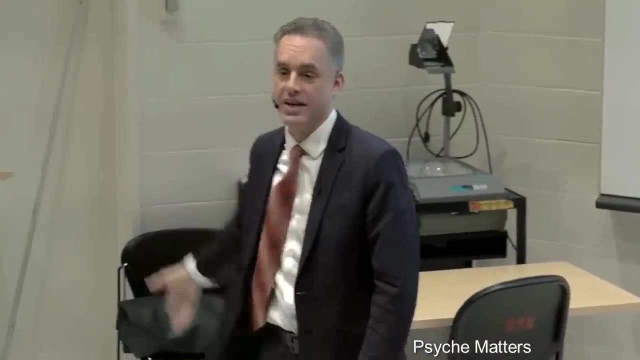 half-heartedly that something good happened to you and they give you a whack and then talk about- you know the great thing that happened to them three years ago Or, worse, the great thing that happened to someone that they knew three years ago. You know it's like go away. 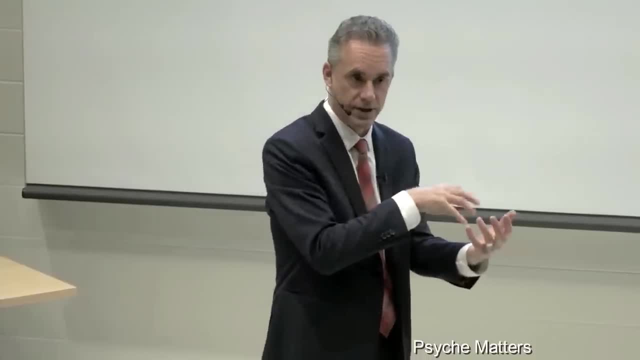 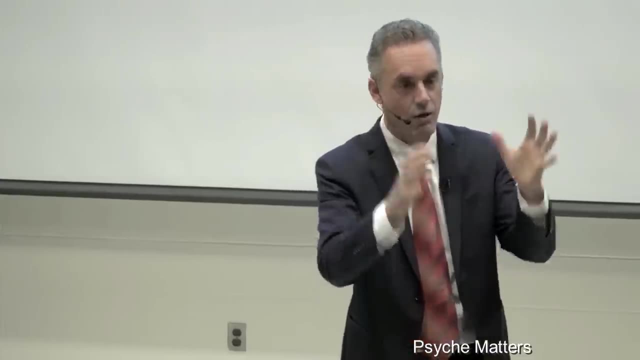 for God's sake. You know they're not helpful to you and they're not helpful to themselves either, And so you want to surround yourself. You've got to think about this. You've got to surround yourself with people who want the best for the best part of you. You can hang around with weasels and losers that are. 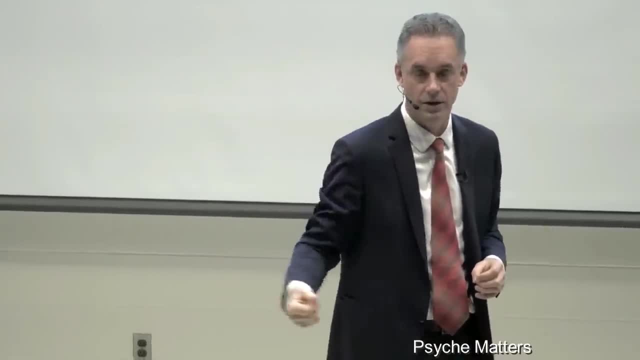 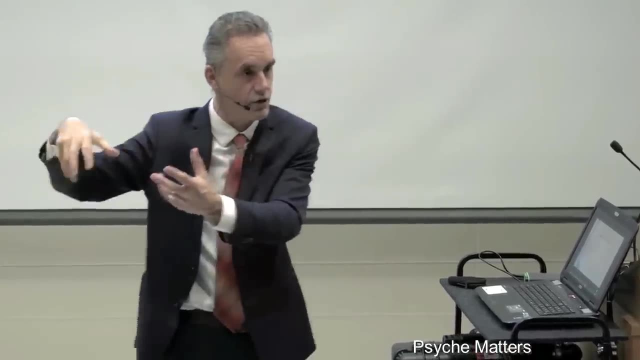 trying to pull you down to justify the fact that they're spiraling downhill as well. And you know the upside of that is you don't have to have any responsibility and you can all whine about how wretched life is, you know. so that's pretty attractive, But I would say it's also a bad. 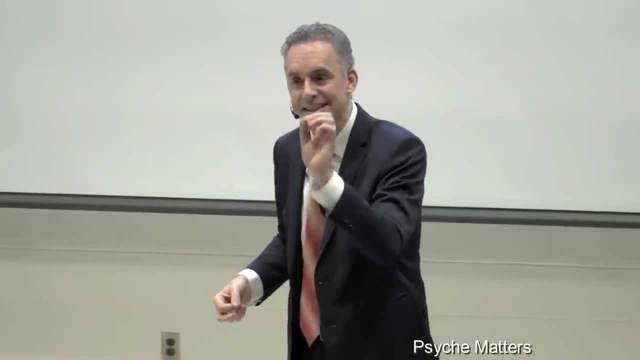 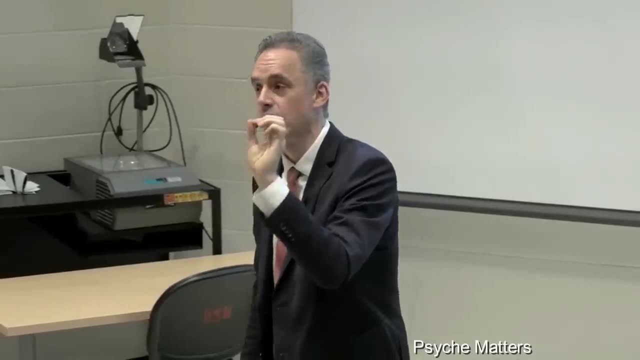 medium to long-term plan, And so it's, it's acceptable and desirable to try to surround yourself with people who are facilitating your development. You know, and you might say: well, I've got people around, I know them well you. 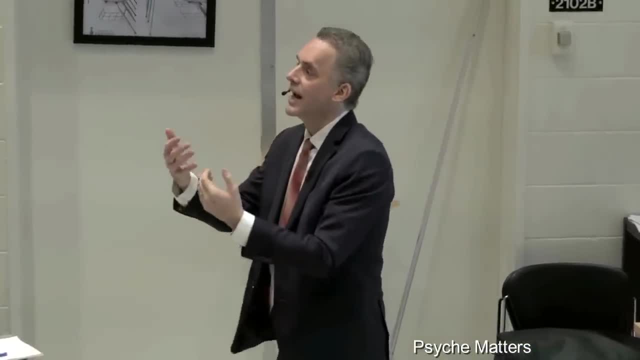 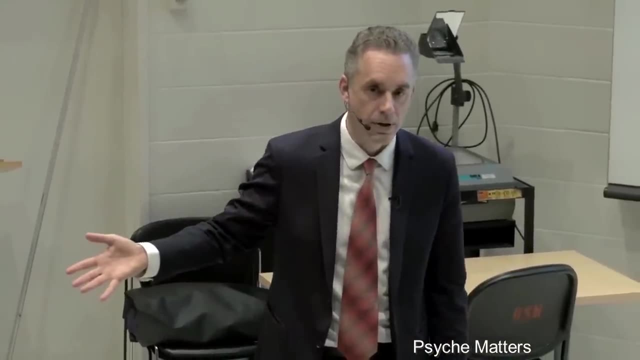 know they're, they're, they're not doing that well, and and they're, and they don't fit into that category. It's like: what's your point? What are you going to do with them? exactly, If they'll, if? 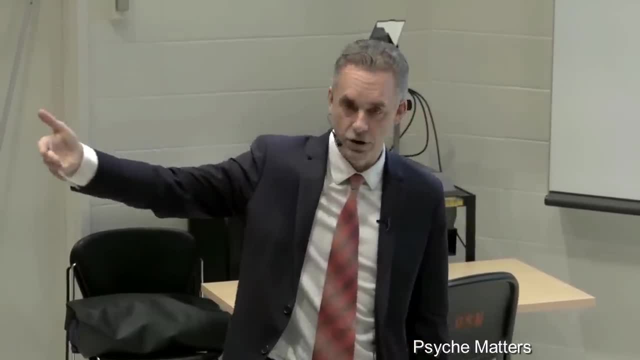 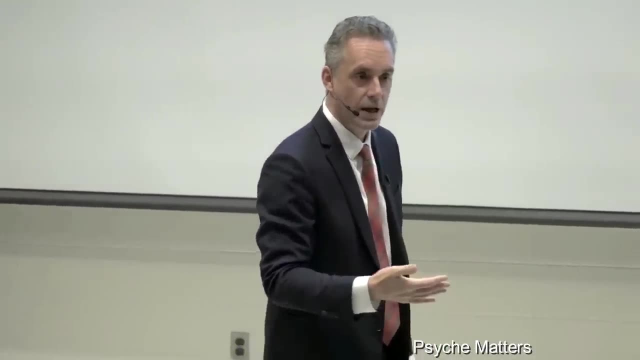 they'll listen and cooperate with you and move towards a better future, great. If they don't- they don't pay any attention and they keep doing the same damn things over and over and they're not going anywhere and it's painful- then maybe the proper thing to do is say: you just have your.